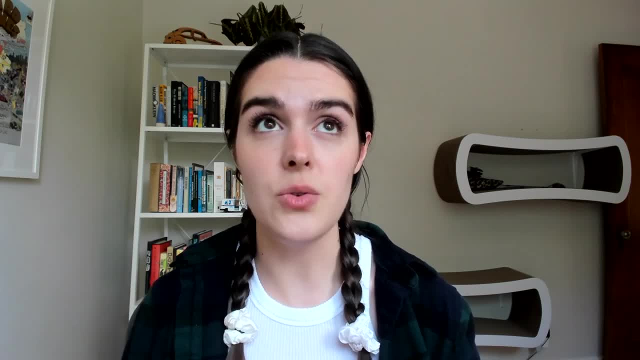 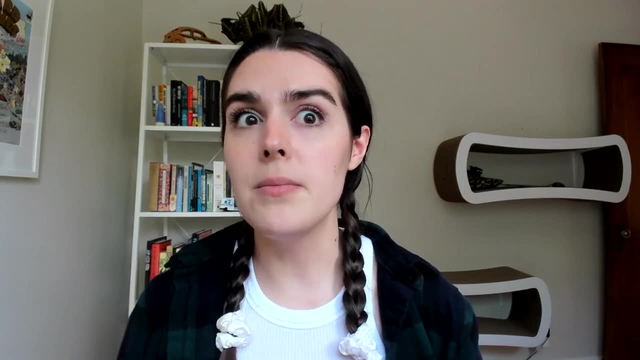 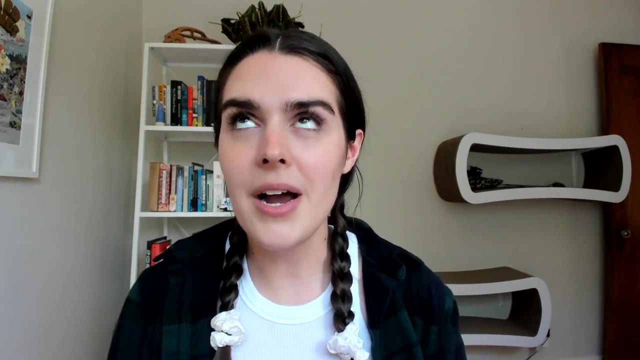 you know that question difficulty has nothing to do with the concept or the topic being tested. So a probability problem can be 400 level or 700 level. A percents problem can be 400 level or 700 level. A prime numbers problem could be 400 level or 700 level. What actually makes a GMAT? 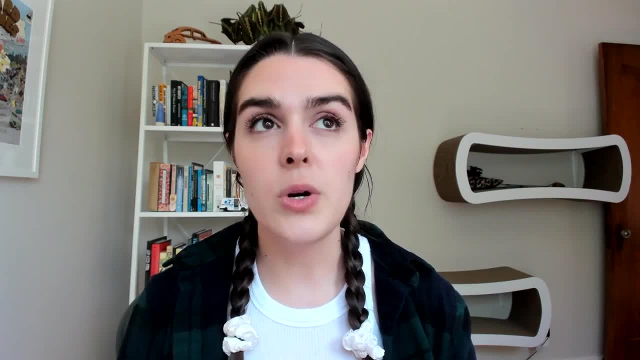 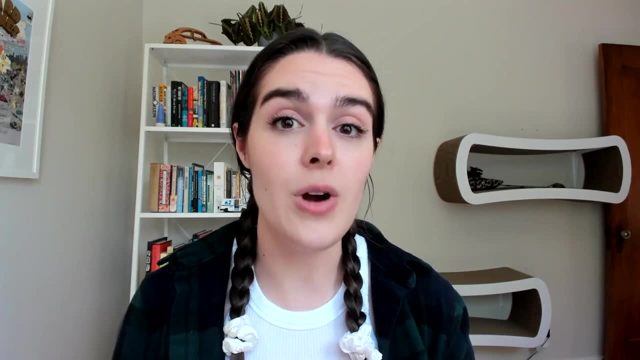 question hard is its complexity, So how it forces you to reason critically, to take more steps, to take less intuitive steps and to avoid traps in order to get to the correct answer. In this video, I want to look at a couple of questions that I think are really important. 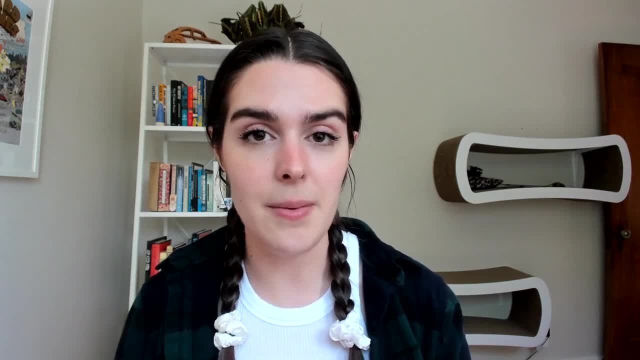 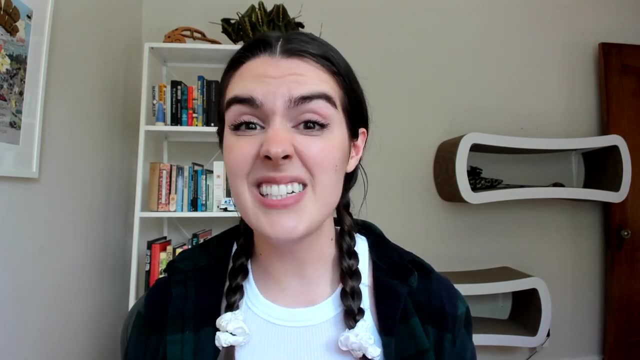 to understand, in order to understand the concept of problem. So I'm going to look at a couple of problem pairs that really exemplify this concept, So one easy to medium difficulty problem and one hard problem that tests the exact same content but at different levels of complexity. 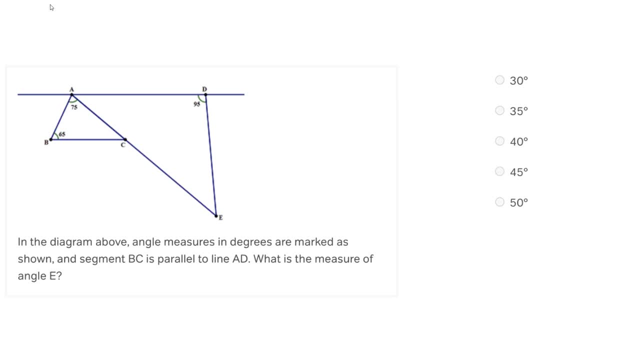 Okay, if you'd like to try this problem on your own, go ahead and pause the video, because we're going to just jump right in. So we've got this diagram. it's got a bunch of angle measurements in degrees, it's got a bunch of unlabeled angles And they tell us that segment. BC is parallel to BC, So we're going to go ahead and pause the video. So we've got this diagram. it's got a bunch of angle measurements in degrees, it's got a bunch of unlabeled angles and they tell us that segment BC is parallel to BC. 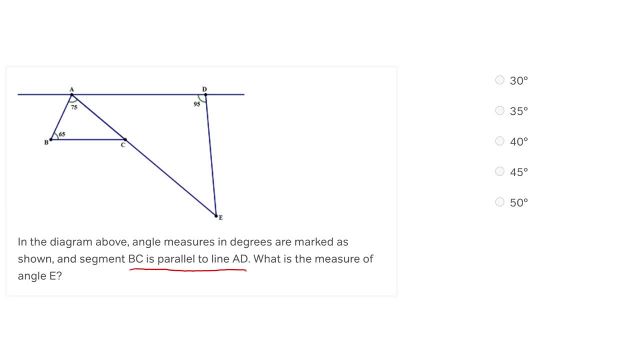 to line a D. that's important. They want us to measure angle E, So I'm going to just go ahead and put a question mark right here to make sure I solve for the right thing. Okay, so, taking a look at this, we've got parallel lines, which means we might be dealing with some lines and angles rules. 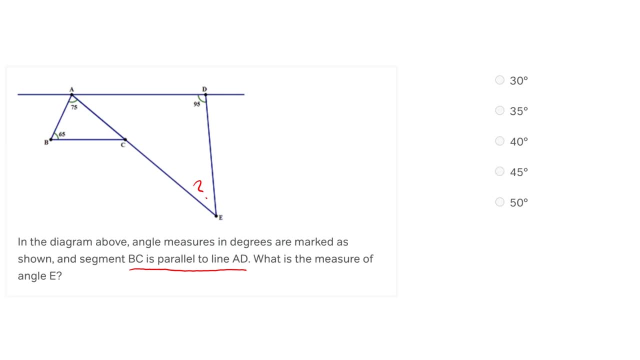 we also can see a bunch of triangles, which probably means we're dealing with the fact that the angles in a triangle add up to 180 degrees. Now, if I just start labeling things, I know I'm actually going to get off to a. 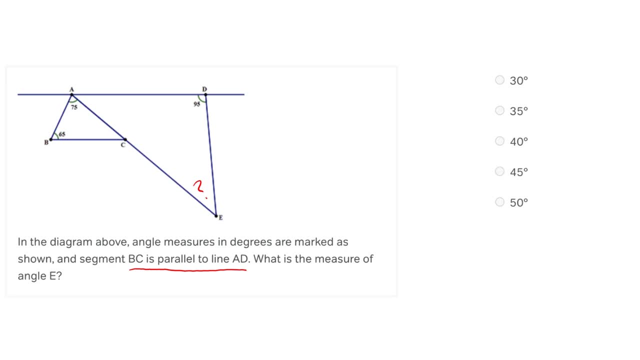 really good start on this problem. So I'm going to go ahead and start with a smaller triangle. So I see that I've got the angle 75 and 65, which means I can solve for the other angle, knowing that all of these should add up to 180.. This should be 40.. Okay, well, using the fact that BC. 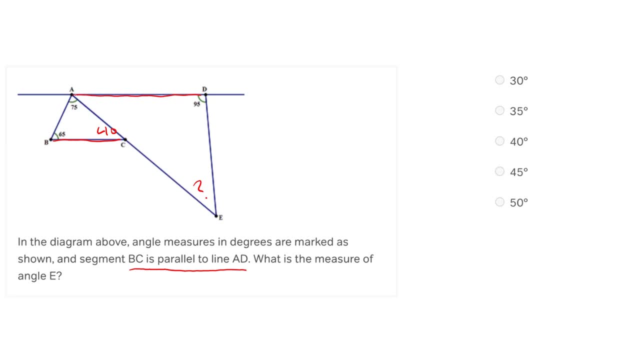 and AD are parallel. we can see that they make this Z shape. So we've got two parallel lines intersected by another line, which means that the angles created by that line are going to be the same as well. So we're going: okay, that is 40,, that is 40. Now 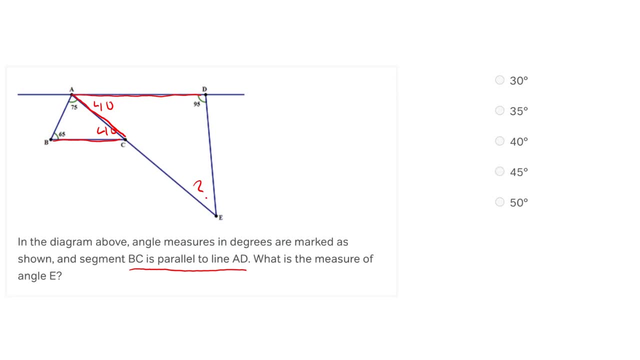 turning our attention to the larger triangle. now I've got two angles in that triangle, which means I can solve for the third. So if I've got a 40 degree angle and a 95 degree angle, that means that I have 135 degrees so far, which means I have 45 degrees remaining. 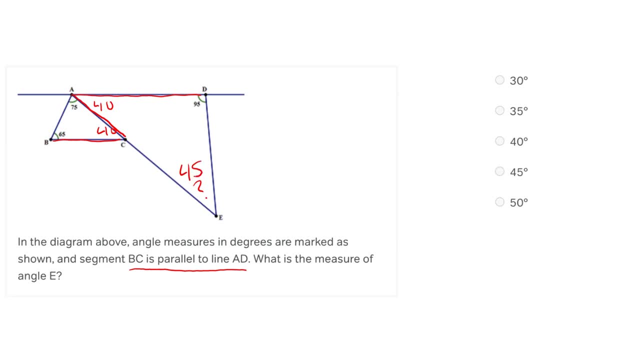 which means the angle that I'm looking to solve for is 45 degrees, And my answer is D. Now there are a couple of places where we could have gone wrong here If we'd stopped halfway through and just gotten the angle measurement 40, we can see that that. 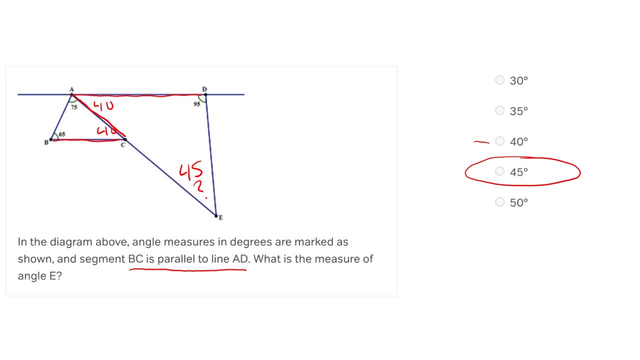 is an answer choice. We could have also made the mistake of adding wrong and ended up with 35. We could have both stopped early and done some math wrong and ended up with either 30 or 50. So there are a couple of mistakes that we can make here, But in general, if we are doing careful. 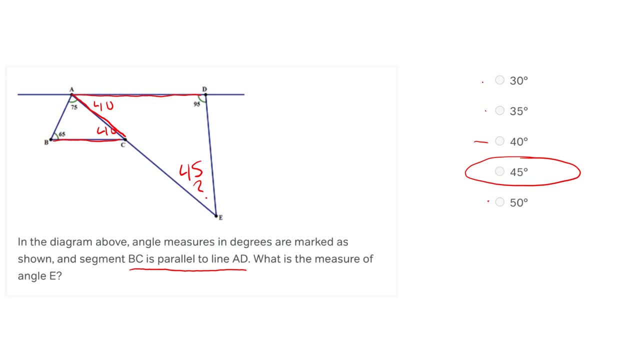 calculation and labeling things on our diagram, making sure we don't stop halfway through. we should get to the correct answer. So this is an easier problem dealing with triangles and lines and angles. Okay, let's go ahead and try a more challenging problem based on the same concepts. 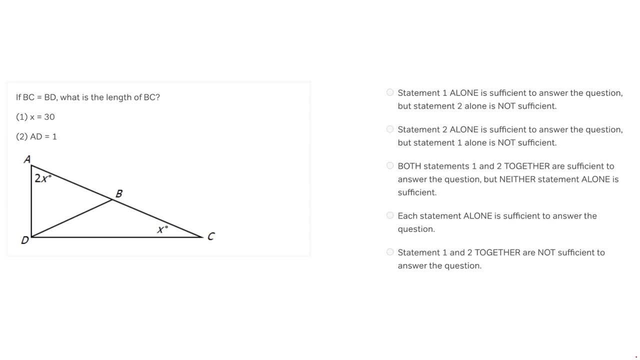 So right away we're going to notice that we've got a triangle that's actually divided up into two triangles. So we know that we could be dealing with some triangle principles here And, as always when we have geometry, we can be dealing with lines and angles. 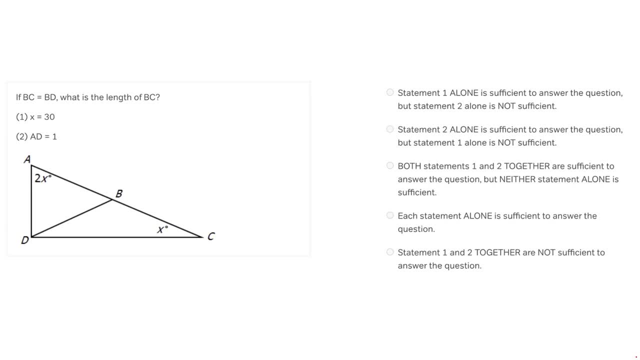 But I'm going to notice here that I have some algebra, So instead of giving me numbers in the diagram, it gives me variables. That's a little bit trickier, And it's giving me a data sufficiency question which automatically kind of lends itself to more challenges and how we approach the. 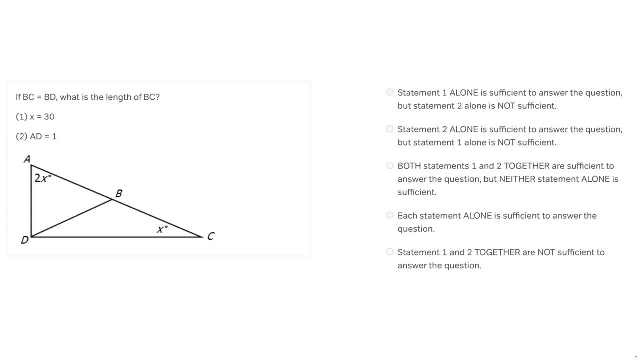 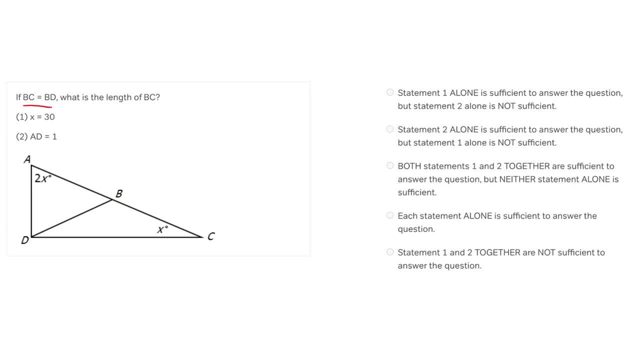 So let's go ahead and jump in with the question stem. We know that BC equals BD. I'm going to go ahead and label that And I'm looking for BC, so I'm going to label that as well. All right now, at this point, maybe the more natural thing to do is immediately jump into 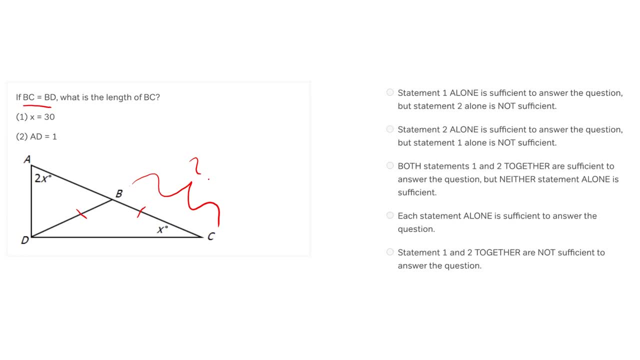 those statements. But I'm not going to do that. I'm going to hang out with this information a little bit more first, to make sure that I really have a solid foundation as I head into the statements. So if I know that BD and BC are equal. taking a look at my 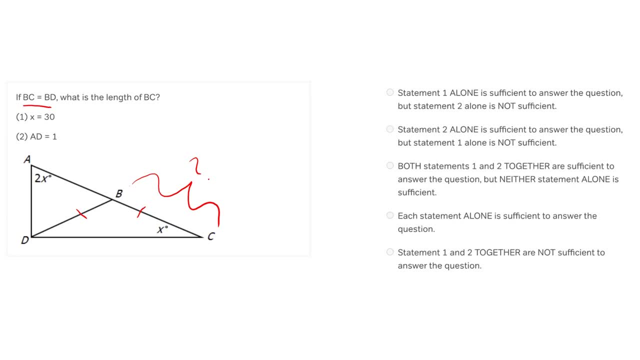 look at the smaller triangle, BCD, the triangle kind of to the right. I'm going to notice: okay, if those sides are equal, that means the opposite angles are going to be equal, which means this angle right here is going to equal X. Continuing to look at the smaller triangle, I know that all 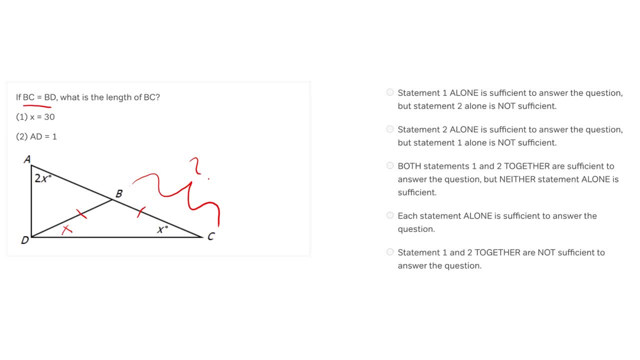 of the angles in that triangle should add up to 180, which means that the other angle in the triangle has to equal 180 minus 2X. Okay, we're still not done. Taking a look at this line here, all right A to C- I know that a straight line is going to add up to 180 degrees. So now I'm 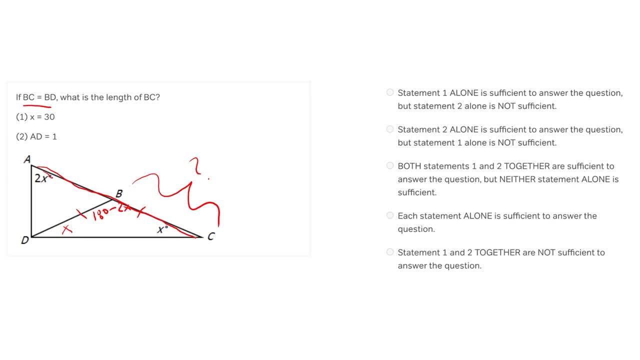 getting my lines and angles. Okay, if I know that this angle on B is 180 minus 2X, that means the other angle on B has got to be 2X Again in order for it to add up to 180 degrees. Now turning my attention to the other smaller 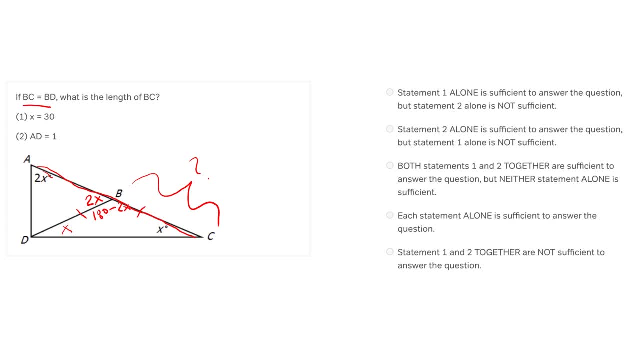 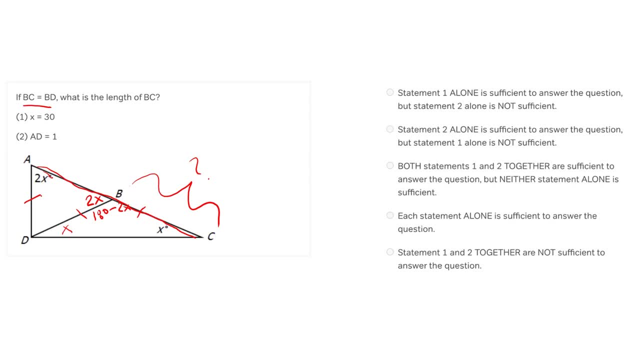 sides are the same. Now, if I've glanced at my statements, that should lead me right to statement two. All right, so that's actually where I'm going to start. I'm not going to start with statement one, I'm going to start with statement two, because I know exactly what I can do with it at. 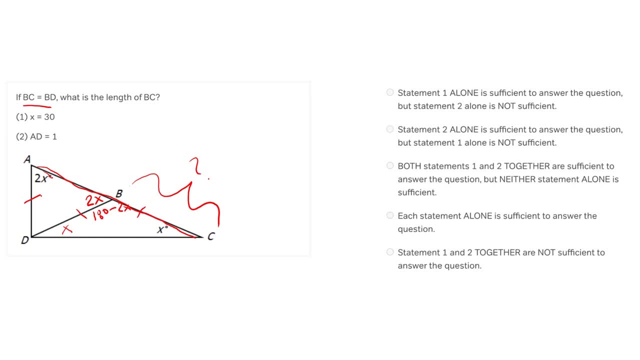 that point. If AD is one, I know then that BD is also one, which means that BC is also one, And that's going to be the same. So I'm going to start with statement two. I'm going to start with statement two. I'm going to start with statement two, I'm going to start with statement one, And 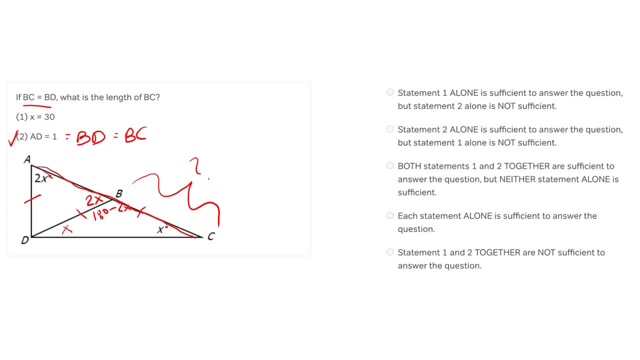 that is what I'm solving for. So I know that statement two is sufficient on its own, without statement one, which means that my answer is going to be either B or D. Now, at this point, I can attack statement one. Now I do not know any of the stuff from statement two. 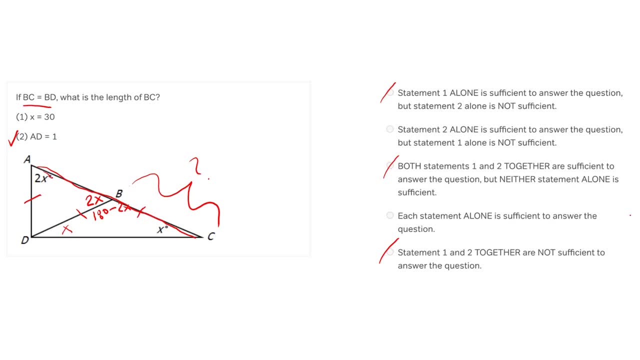 So I do not know what those sides actually equal, but everything else that's on my diagram I do know, because that was from the question stem. Okay, so at this point I know that all of my X's are 30 degrees, So that means that I could fill in all of these. 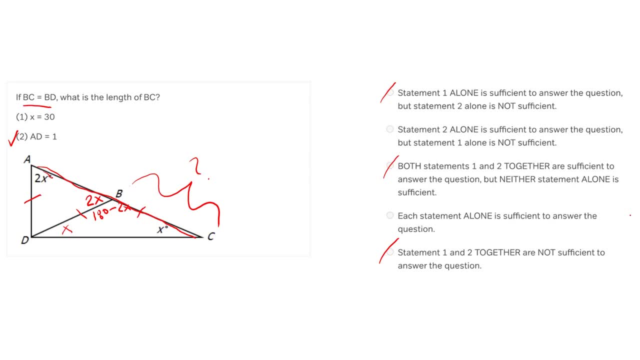 different angles. I can find out every angle in this triangle successfully And that's going to tell me that this larger triangle is a 30,, 60,, 90. It's going to give me a lot of great cool information. But before I do too much of that, I want to think logically for a second, Even if I 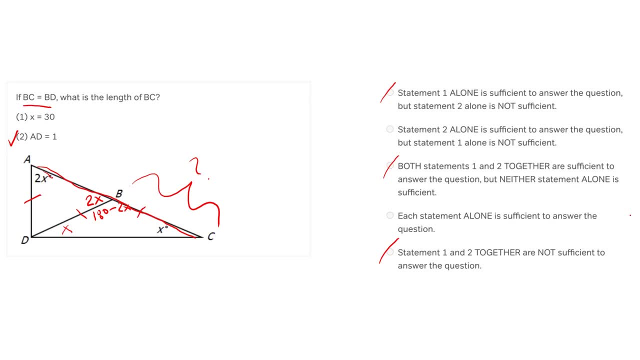 know all of the angles in the triangle, I'm not going to be able to find out every angle in this triangle And, as a result, know the ratios of the sides in the triangle. That doesn't give me any information about the scale of the triangle. So even if I do know all the angles, there's no way. 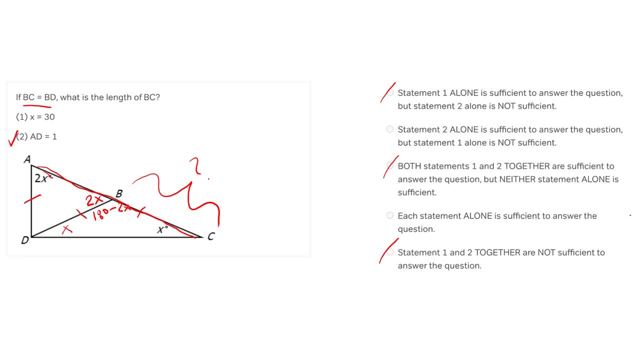 I'm going to be able to figure out the side lengths. So statement one on its own not sufficient, And the answer here is B. Now, because we approached the problem in this way, we were able to get to the answer. But let's talk through a couple of ways we could have gone through this. 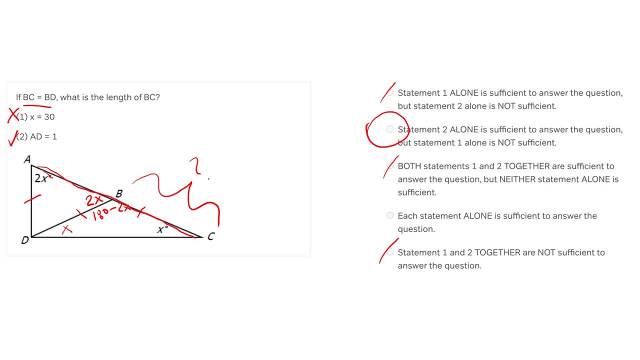 wrong here? We could have started by starting with statement one. When we start with statement one, we learn about the angle relationships, And that tells us about the relationships between the sides, which then, when we look at statement two, really goes: oh, and now I know something about. 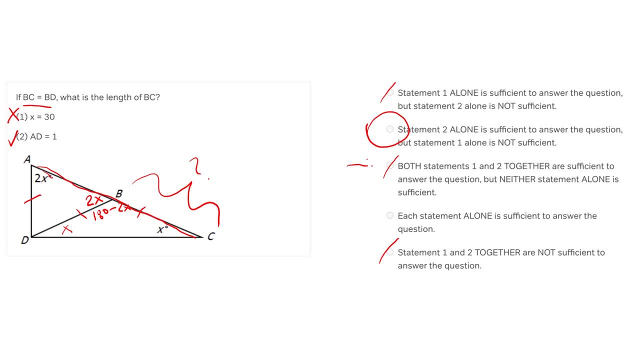 the sides. So together I'm going to be able to solve. And that leads us to C. Now, this is a flaw in thinking about data sufficiency, where we put the statements together before we think about each of them individually. So we would have just said: oh, I don't know, I don't know, I don't. 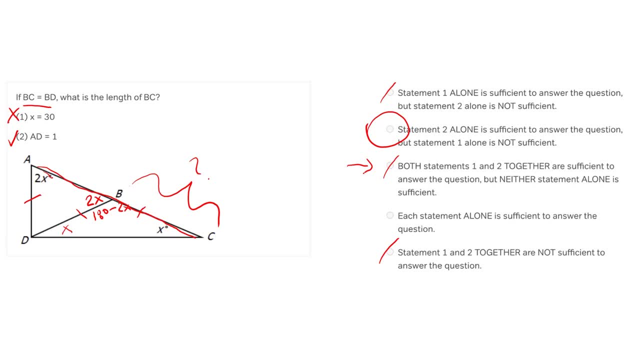 know I just skipped trying to solve for statement two. on its own That's a trap. The other thing that we could have gone wrong with here is not being able to put together all of the different relationships in this diagram, So there were more complex relationships here between the various 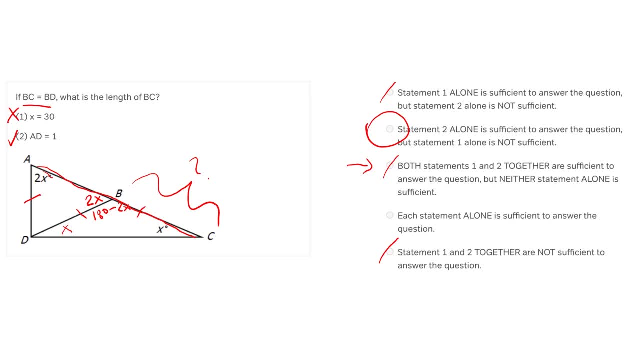 lines and angles and the various triangles than there were in the other problem And they were algebraic rather than just basic values. So same exact concepts, triangles, lines and angles, but they were not able to put together all of the different relationships in this diagram. 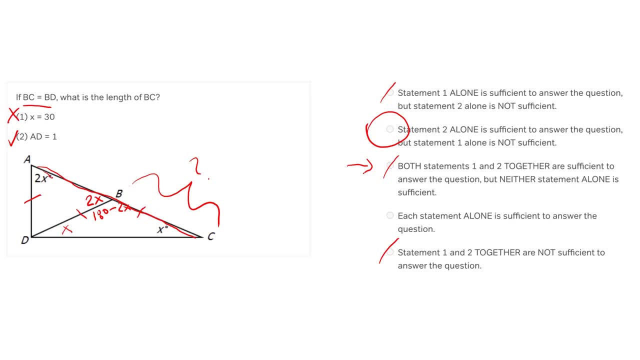 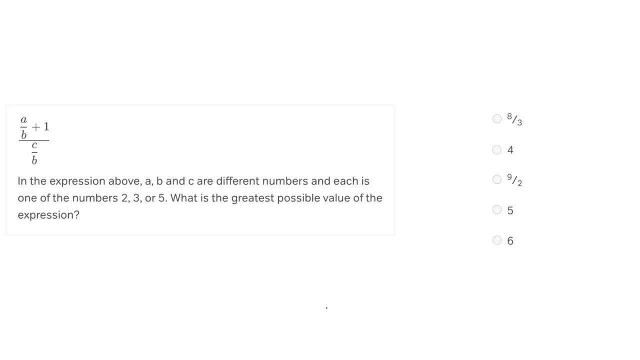 So we're going to have to test it in a more difficult problem that requires us to use this knowledge in a more unintuitive way. Okay, let's try another problem: pair. So in this problem we have this expression with A, B and C, And A, B and C can be two, three or five, So it could 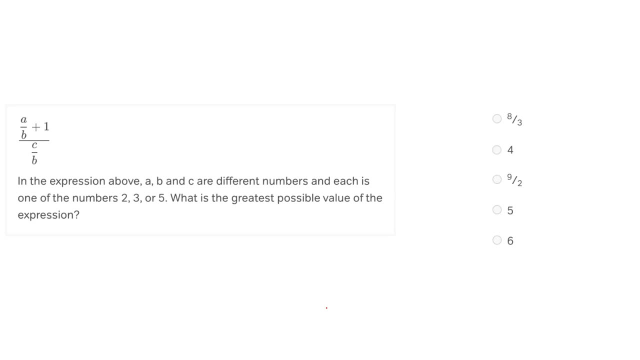 be A is two, B is three, C is five or C is two, B is three, A is five or some other mix and match version, And we want to find the greatest possible value of A, B and C. So we're going to have to. 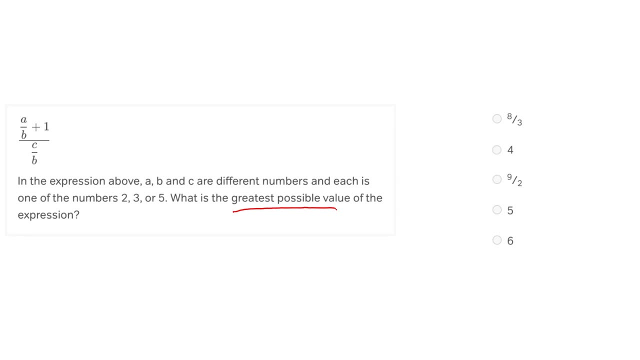 use the expression of the expression. Okay, Now, this is not an easy problem, in the same way that the first problem was, because there is a kind of natural way to approach this which is just plugging in the numbers until you get the highest possible value, And that's going to be slightly. 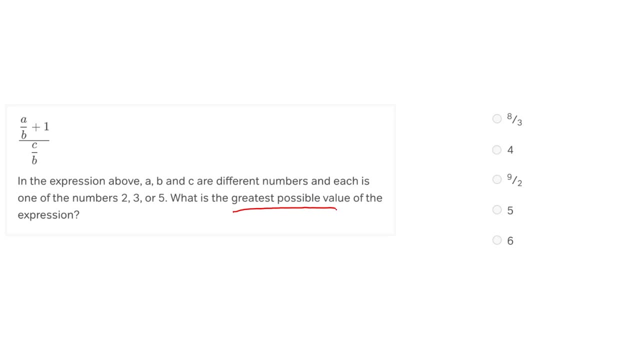 less efficient than the way that we're going to solve it. So the kind of natural course of action is probably not the best option here. So that makes this maybe more of a medium problem. However, if we're going to use the expression of A, B and C, then we're going to have to use the expression of 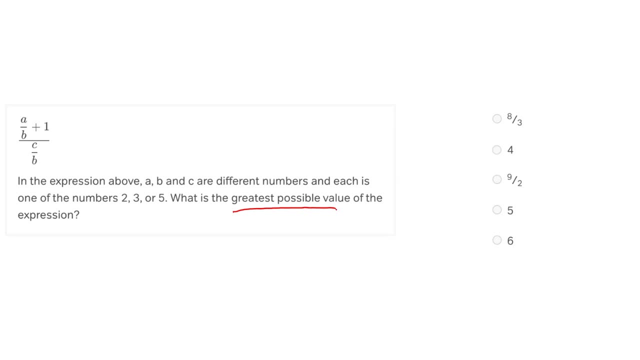 A, B and C. So if we take a little bit of time with this question stem and with this expression, we're going to be able to solve this relatively efficiently. So first thing I'm going to notice is that this expression is not in a super convenient form. Fractions and fractions. 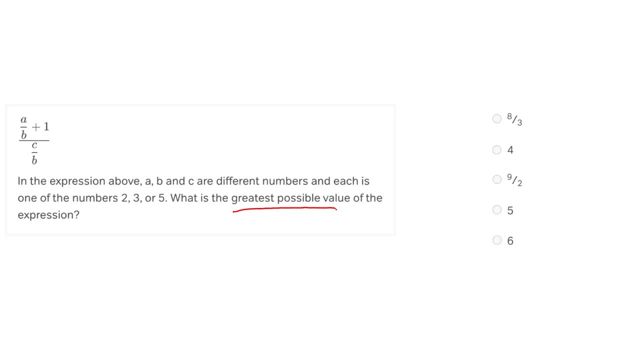 kind of gross. So instead of dividing by a fraction, I'm going to multiply by the reciprocal. So really, here I have A over B, plus one times B over C. Okay, Now at this point I can go all right, I have this addition here and I don't love that, right. But I know that when 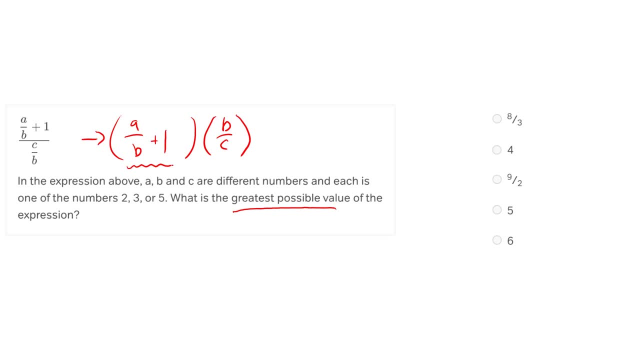 I want to add two things, and one of those things is a fraction. I'm going to need to get a common denominator, So I'm going to multiply by one on this one, by doing B over B, and that will give me a common denominator. So I really have A over B plus B over B, which will allow me to rewrite this. 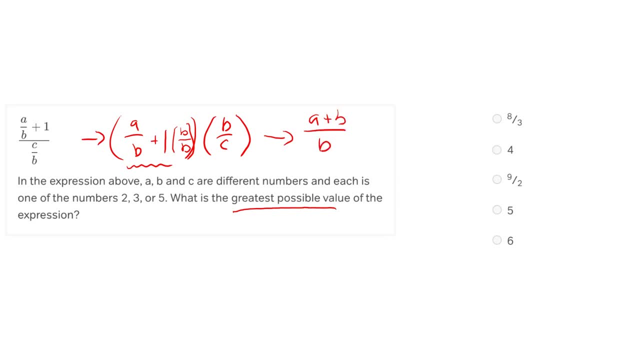 term a plus b over b, and again that's going to be times b over c. Now we see the magic. So because we've got a- b in the denominator and a- b in the numerator, those b's cancel and we have a plus b. 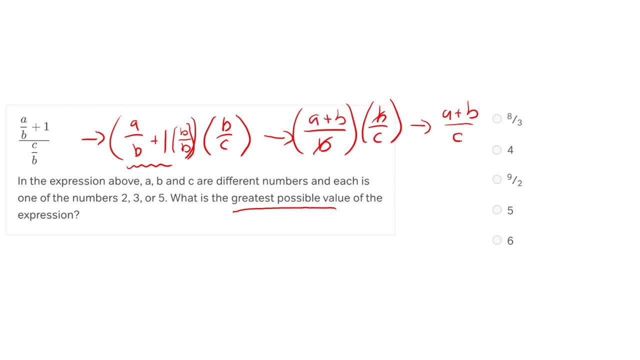 over c. Now how we want to approach these values is going to make a lot more sense. So I definitely want my larger ones in the numerator and my smaller ones in the denominator so I can get my greatest possible value. So I'm going to put 3 and 5 up top 2 in the denominator so I get 8. 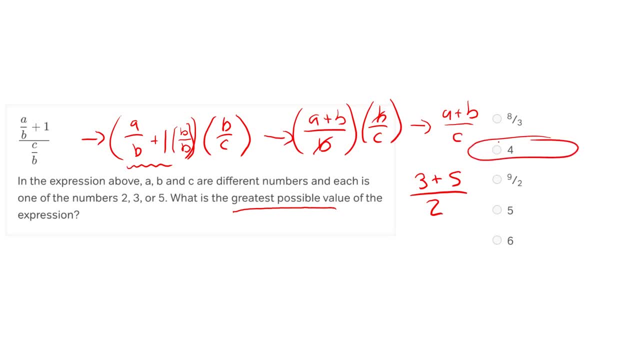 divided by 2, and the answer is 4.. So once again, we can go kind of an incorrect route here and just start plugging in numbers- and that's what's going to lead me to these other options- is just plugging them in in a less than ideal way or potentially doing some bad math. But if we take a little bit, 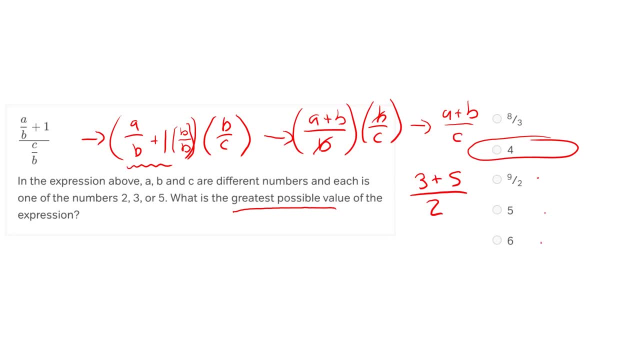 of time. to simplify this, this problem again leads pretty naturally to the correct answer. So not easy, but maybe more of a medium level. So this problem tests concepts of arithmetic, really understanding the operations specifically of multiplication and addition. Okay, let's go ahead and try a harder problem that tests the 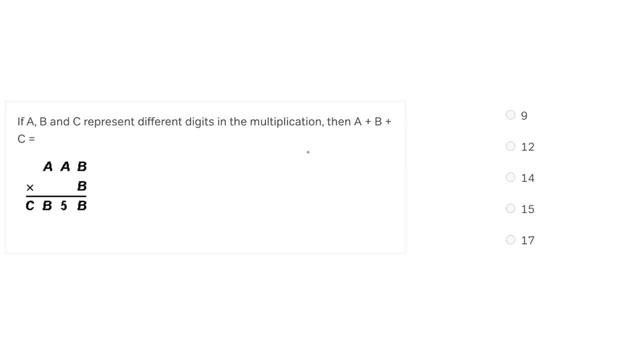 same concepts. So right away we can see some similarities in this problem. with the last one, We have three unknown variables that represent different digits and we're trying to solve for an error Arithmetic expression. Now a couple of differences. We are trying to solve for an. 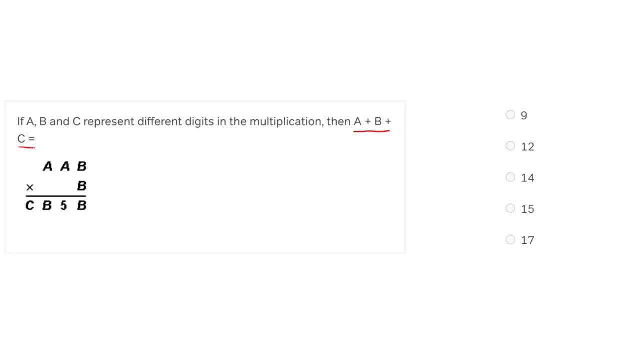 arithmetic expression, but rather than the greatest value of that arithmetic expression, we are solving for the only value of that arithmetic expression based on this arithmetic equation, right here. Similarly, instead of having the options of 2,, 3, and 5 to choose from, 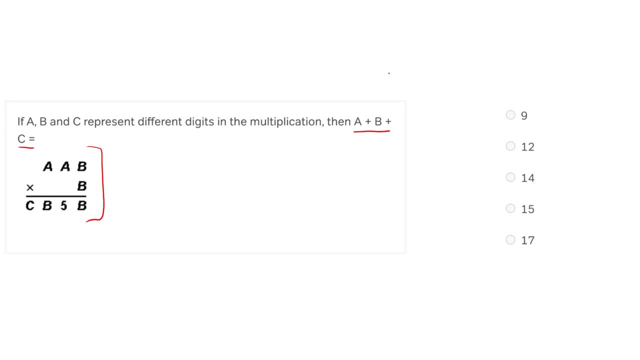 we have any different digit, So we can work with 0,, 1,, 2,, 3,, 4,, 5,, 6,, 7,, 8, or 9.. So a lot of options Worth noting at this point that on the previous problem. 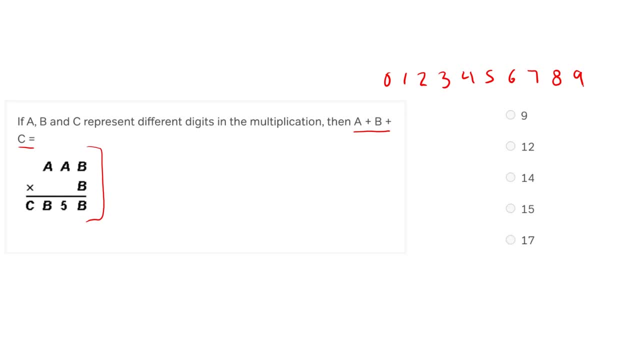 we could have solved by plugging in the different numbers and then just trial and erroring until we got to the right one. However, with this problem, that is not going to work. There are just going to be too many options for that to be a viable course of action. So this problem is harder. because not 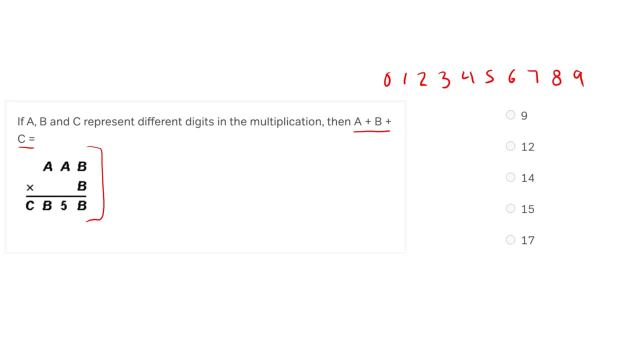 only would it be slower. it would be so slow as to be impossible with this method. So we are going to need to implement our knowledge of multiplication and addition in order to solve this correctly. Okay, so, coming back to this equation, So we have a three-digit number times. 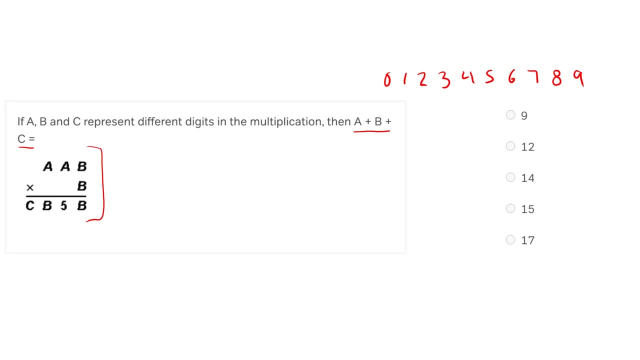 a one-digit number, that gives us a four-digit number. We also notice we have four different B's, so those all have to be the same digit, and two A's. those also both have to be the same digit, And that gives us some clues for where to start. So, taking a look at our ones place, 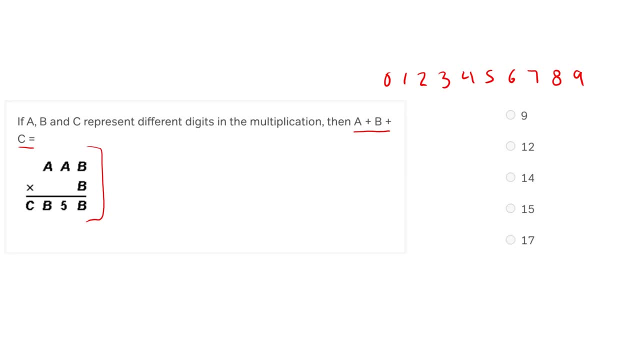 we notice that we have a three-digit number times a one-digit number. So we have a three-digit number times a one-digit number. We also notice we have a B times a B. that's going to give us a B. So B times B is going to give us some number that ends in a B. Okay, well, there actually aren't a lot of. 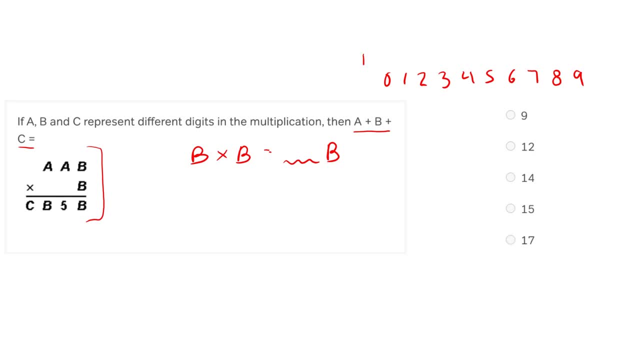 digits that are going to make that work. So we can actually go through our options and start narrowing down. So starting with zero. well, zero times zero is technically zero, so that would work here. But if we take a look at the problem, a three-digit number times zero is going to be zero, not a four-digit. 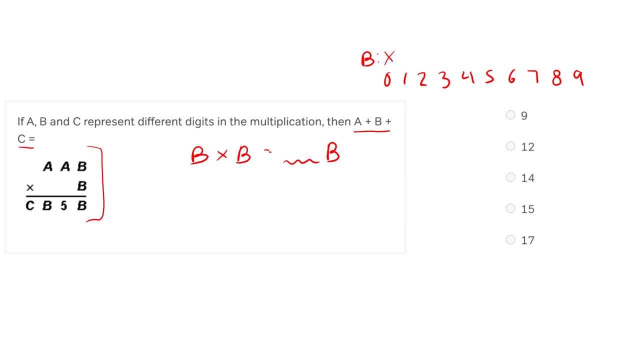 number, so that's not going to work. Same deal with one One times one technically does end with one, but a three-digit number times one is going to give us a three-digit number, not a four-digit number. Nope, All right, two times two. 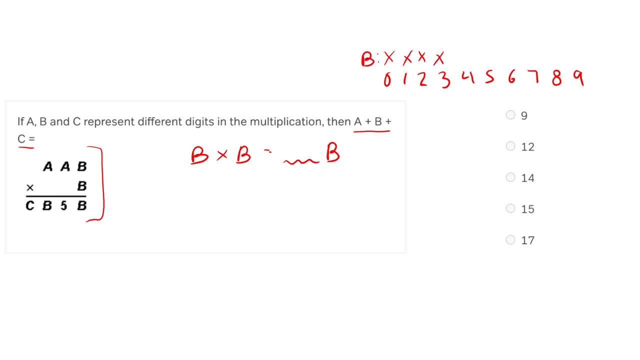 is four. Nope. Three times three is nine. Nope Four does not work. Four times four is 16.. Five times five is 25.. That does end in a five. That's an option. Six times six is 36.. That's an option. 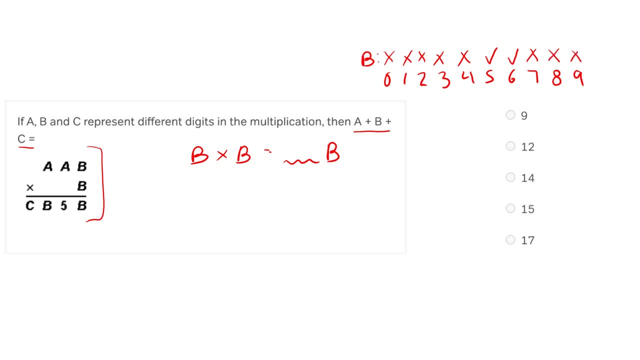 If we do the same process for seven, eight and nine, those don't work. Okay, so let's go ahead and try our options. So starting with five, so five, five, five, five. Okay, so five times five is 25.. Carry the two. 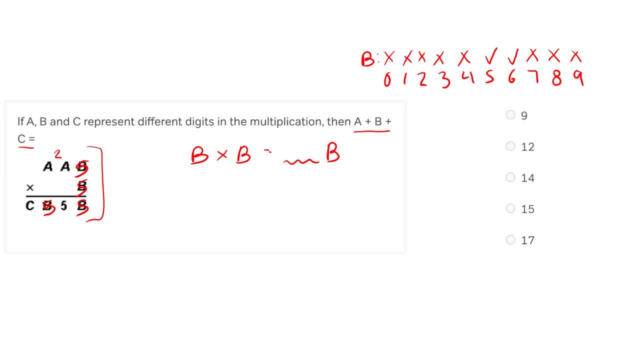 And then this is where the problem starts to get even harder, because now we're dealing with some slightly more complicated arithmetic. So if we were to be doing this problem, we would do five times a and then add two to get something that ends with this five. Okay, I'm going to write. 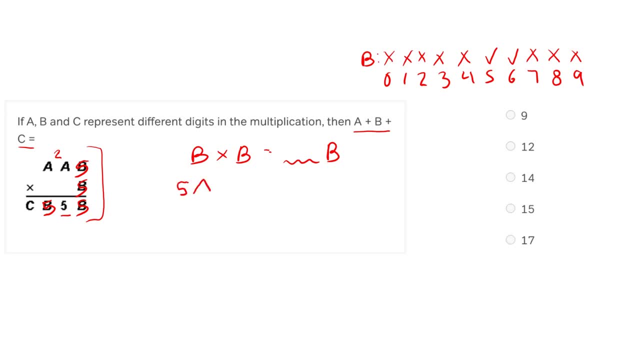 that as its own problem once again. So five times a plus the two that we carried should give me something that ends with five. Okay now, I can actually manipulate this by subtracting two on both sides, So I get five. a is going to be equal to something that ends with a three. Okay now. 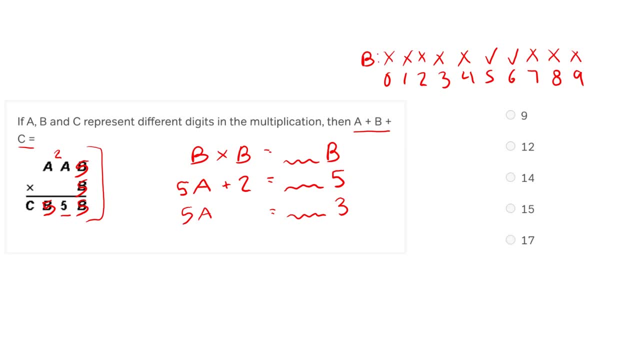 hopefully. at this point I can see that that's not going to work. Five times anything is going to end with a zero or a five Again, any integer, So it's never going to end with the three that we want. So we're going to write that as its own problem once again. So five times a plus the two. 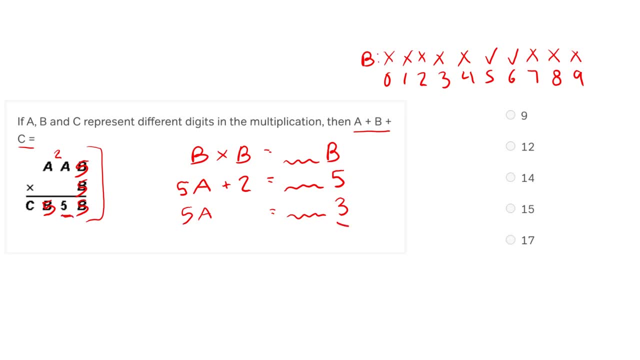 in order to add the two, to get the five that we want Complicated. But in other words, the b cannot be a five because it would make our a an impossible number. So that means b has to be six. We know that, Okay, so let's try that. All right, so b is six. 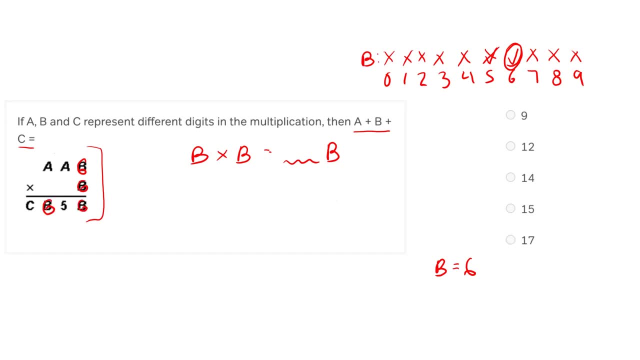 Filling that in everywhere. All right, six times six is 36.. Carry the three And once again we have similar math. Six times a plus the three that we carry should give us something that ends with a five. Manipulating that by subtracting three on both sides, we know that six a is going. 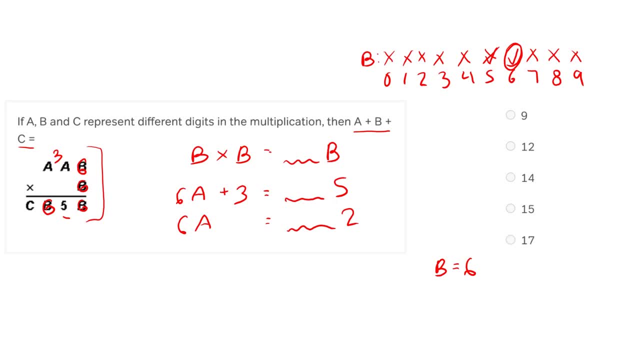 to have to end with a two. Now there are actually some options that will work here, So trying out a. okay, we know that a now can't be six because we've already used that one, So we're going to use that option. Six times zero is zero. Six times one is six. Six times two is 12.. That could work. 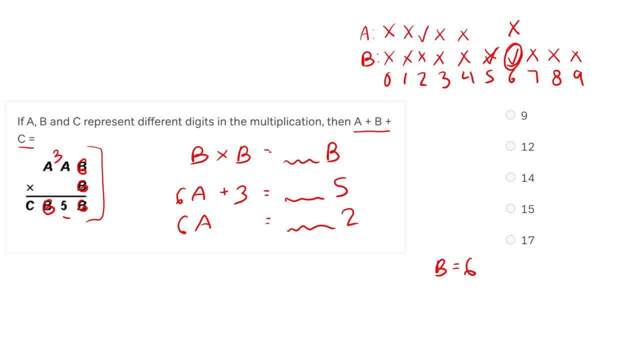 That ends with a two. Six times three won't work, Six times four won't work. Six times five won't work. Six times seven is 42. That could work. And then eight and nine won't work. Okay, so again. 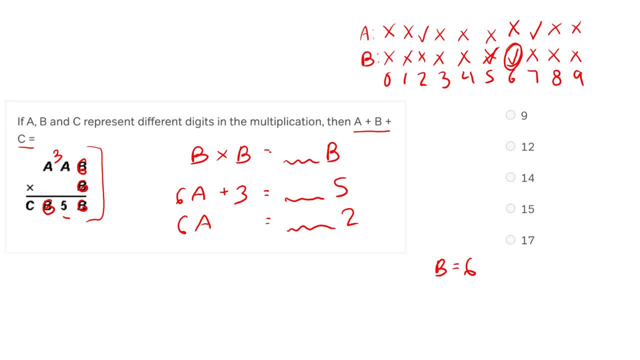 we have two options. We're going to try them both. Okay, so, starting with a two, filling in a two for a in both places. Okay, six times a plus the three. All right, so we have six times a plus the three. 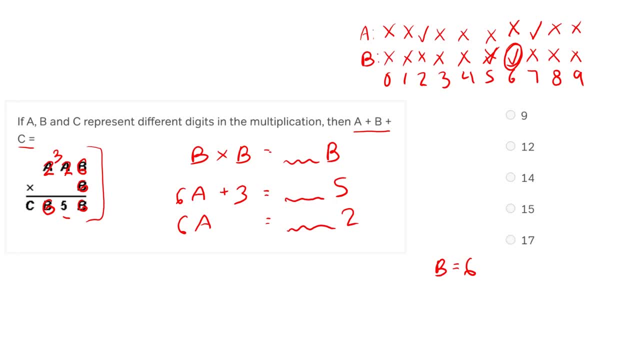 Six times six was 36.. Carry that three Six times two is 12 plus three. It gives us that five down here for 15. and then carry the one right here: Six times two is 12 plus one should give us 13.. 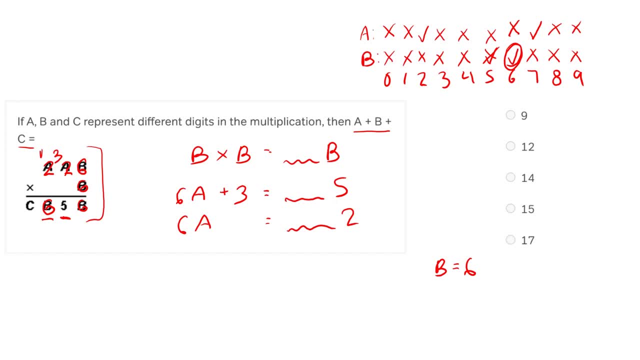 But we got a six right here Doesn't work, Okay. so a cannot be two, It's gonna have to be seven. Okay, we are almost done, So going ahead and getting rid of what I did there. All right, Now I know that six has to be seven, So filling that in. Okay. so six times six was 36.. 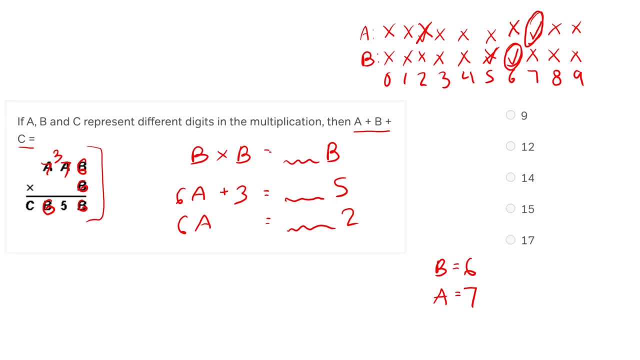 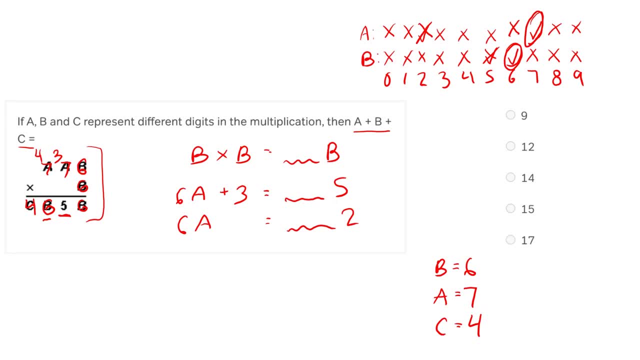 add a four. So I'm going to add a four. So I'm going to add a four. All right, Adding those up for a plus B plus C gives me 17. And the answer is E. So testing the exact same concepts in a seemingly similar problem. Again, this is just arithmetic. 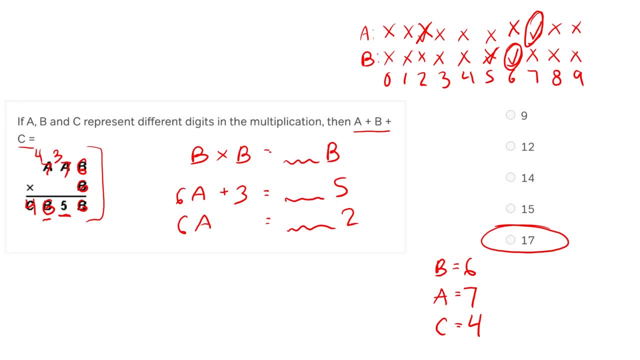 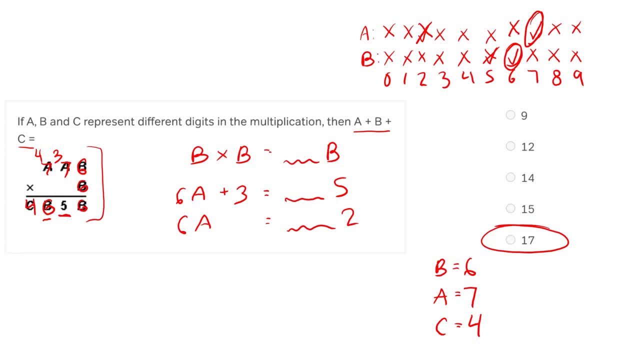